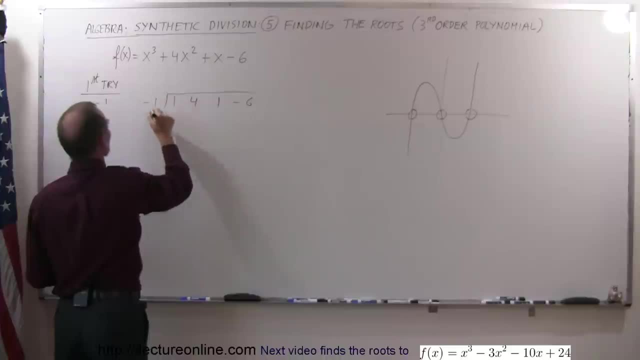 minus 6, my division sign. I use my first try, put the line down here and just quickly go through the maneuver of how to find the roots. we drop the 1 down 1 times. the negative 1 is negative 1. add it together. we get 3. 3 times negative 1 is negative 3. add them together you. 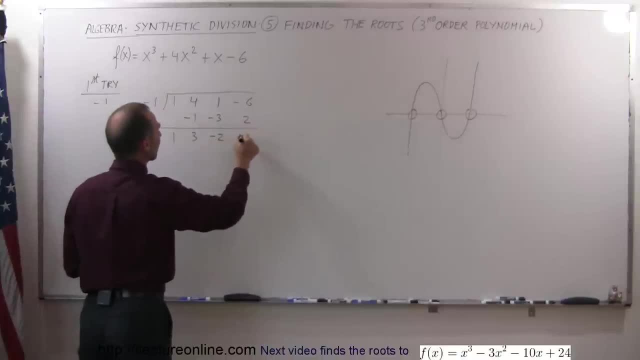 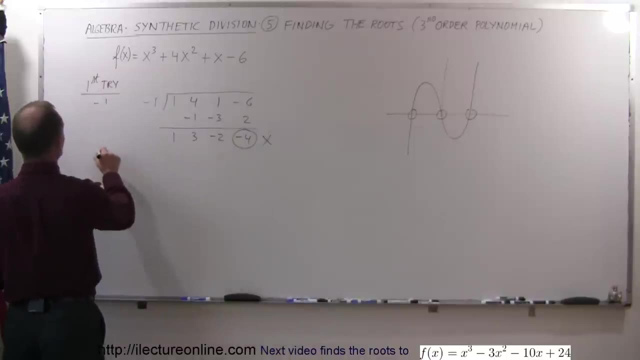 get negative 2, negative 2 times. the negative 1 is 2. add them together, you get negative 4 and you can see it's not 0. so that was not one of the roots. Okay, let's try positive 1 and again we. 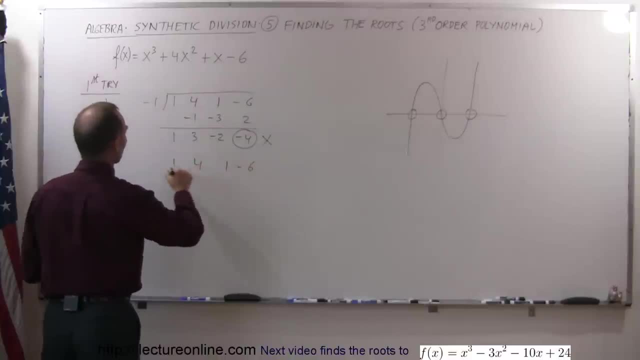 put in our coefficients 1, 4, 1 negative 6, then our division sign. now it's a positive 1. put our line down here. drop the first number: 1 1 times 1 is 1. 1 plus 4 is 5. 5 times 1 is 5. 1 times 1. 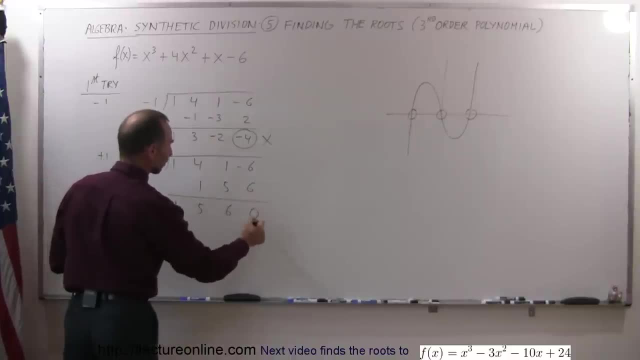 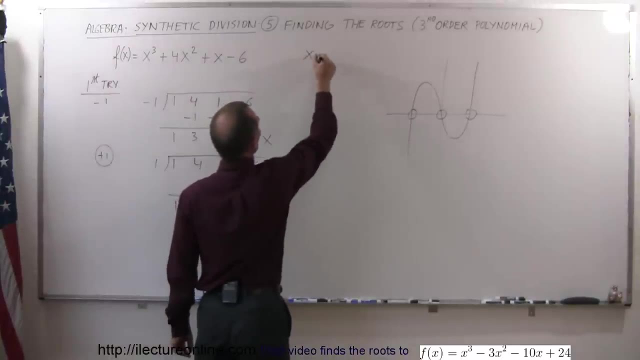 plus 5 is 6. 6 times 1 is 6 and look at that. that adds up to 0 and we say: bingo, we found one of the roots. the root is plus 1. that means x equals 1 is one of the roots and so that means our polynomial. 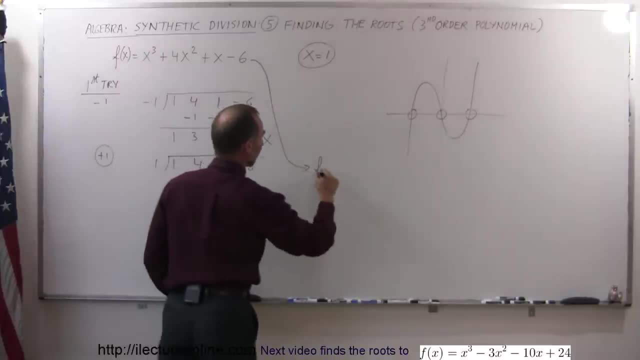 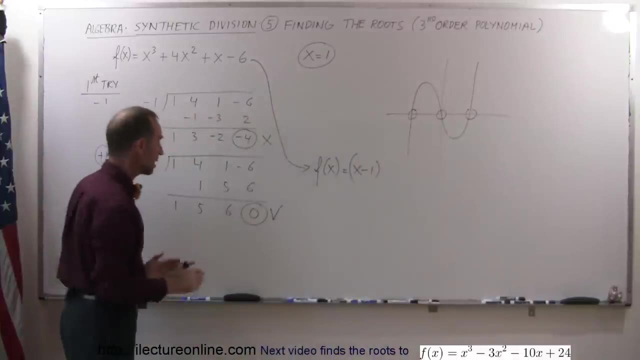 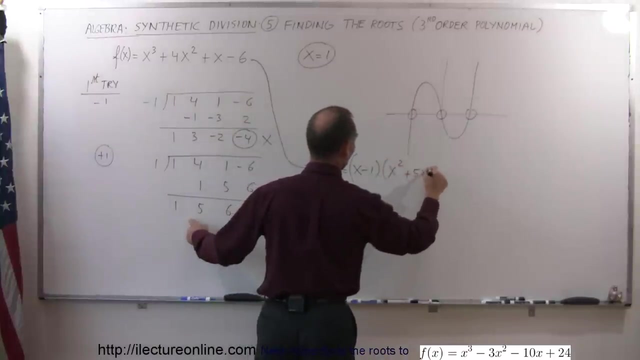 now can be written as: f of x is equal to, since that's one of the roots, and so that means our polynomial is equal to, since that's one of the roots, it would be x minus 1 times what's remaining here would be right. here. that would be x squared plus 5x plus 6, and of course to continue, then we 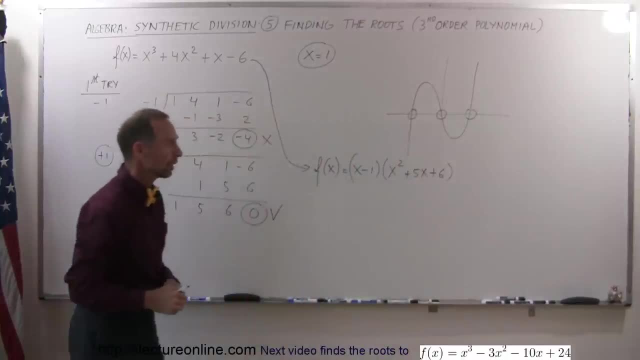 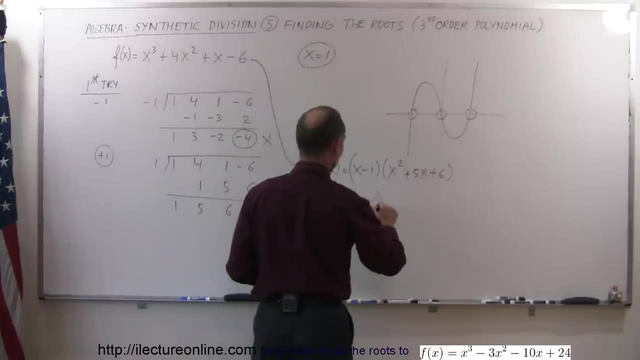 need to find the roots of this part of the polynomial. now that is actually relatively easy because we know how to factor that. so this can be written as x minus 1 times we get an x and an x a plus, and of course I need two numbers. when you add them, you get 5. when you multiply them get 6. 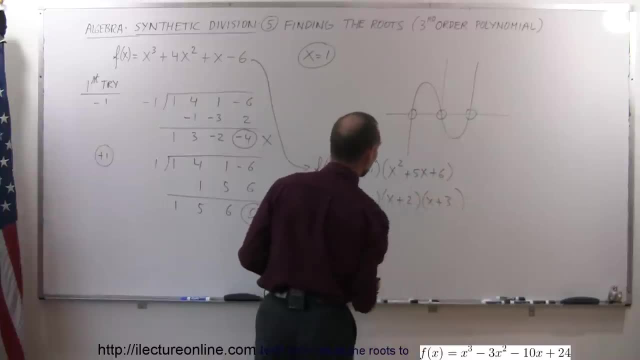 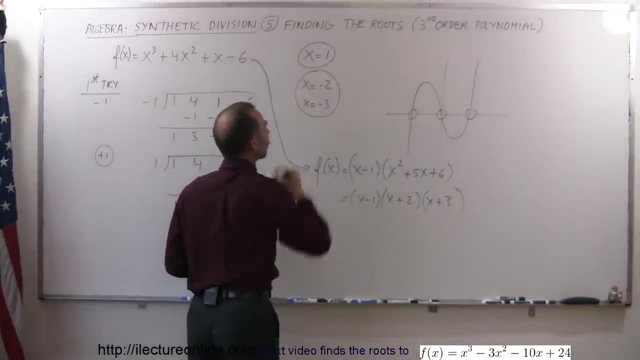 and that would of course be 2 and 3. that means x equals minus 2 and x equals minus 3 are the other two roots. so what's so nice about synthetic division is that the first root that's very difficult to find once you have it down to x minus something, times a polynomial of second order. then 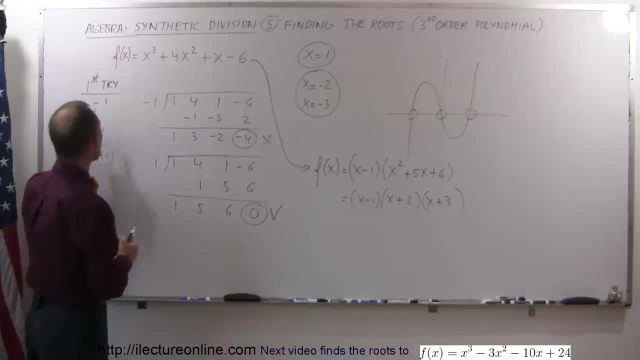 the rest is easy to find, but it's that first root that's hard to find, and using synthetic division, you can see how you can find the root. in the next video I can actually show you how you can actually zero in on the correct root using synthetic division. so I'll show another example next.